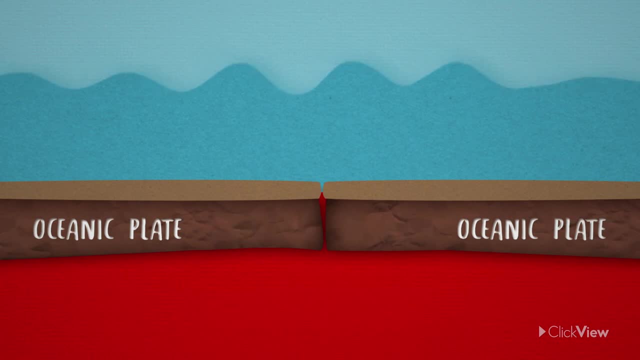 But over time these plates are brought together. time. this allows extremely hot magma to rise up from deep within the planet. Magma rises and fills the gaps created by the plates moving away from each other And eventually new crust is formed. 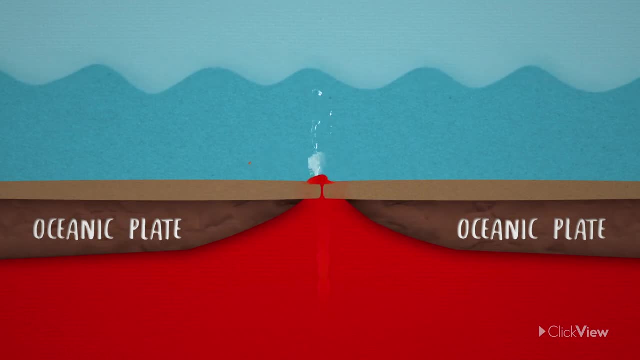 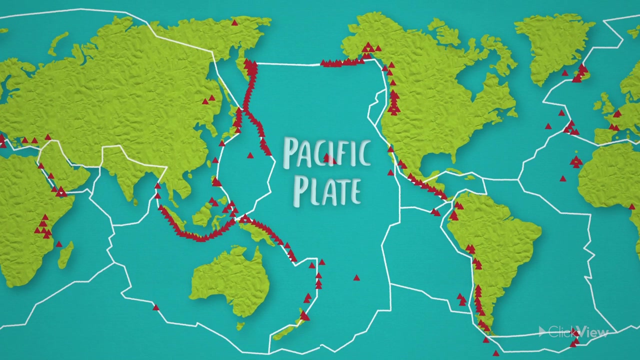 Magma at the margin can sometimes explode through this new crust, creating a volcanic eruption. Many of these constructive margins are found under the ocean. If you map the locations of volcanoes, you'll see that 75% of the world's active volcanoes 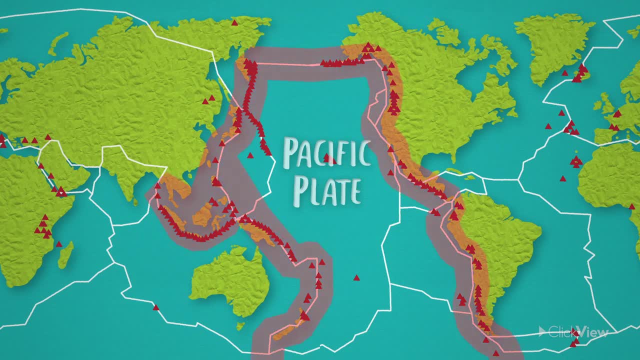 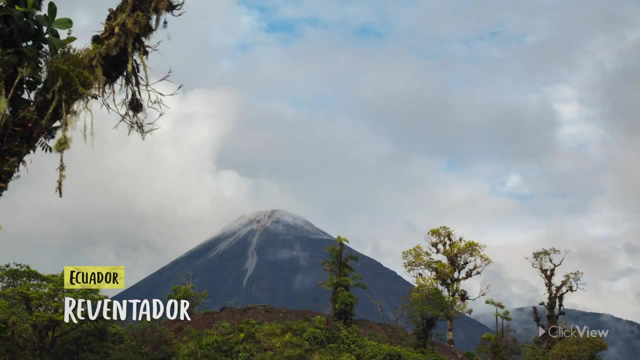 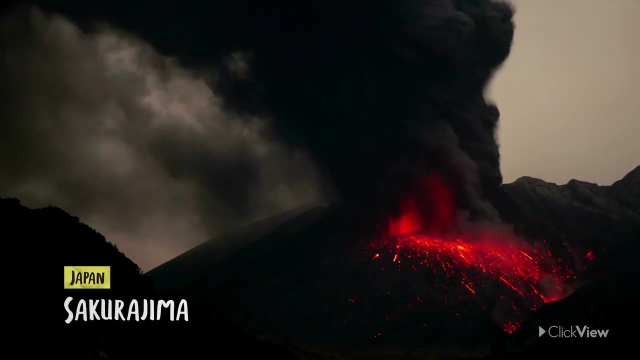 are along the margin of the Pacific plate. Volcanologists refer to this as the Ring of Fire. Since 1850, approximately 90% of the 16 most powerful volcanic eruptions on Earth have occurred within the Pacific Ring of Fire, making it one of the most dangerous places. 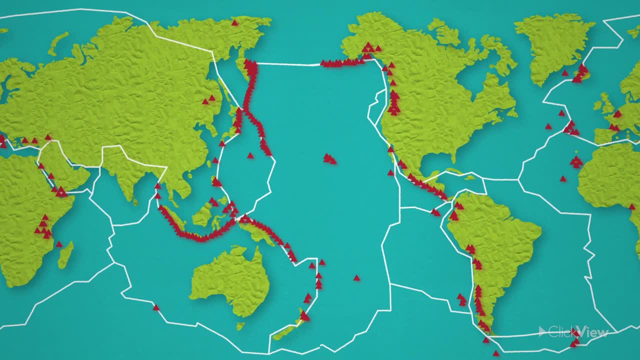 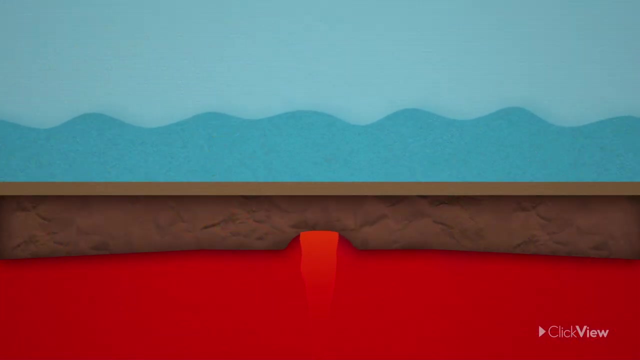 on Earth. However, there are places on Earth where a volcano can form away from tectonic plate boundaries. We call these hotspot volcanoes. They form when rising magma from deep within the planet melts through the tectonic plate above and begins to build up. 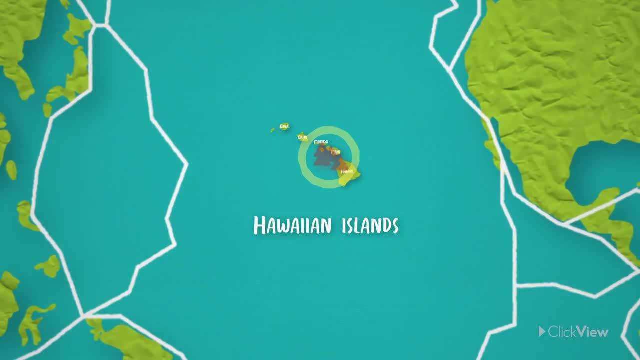 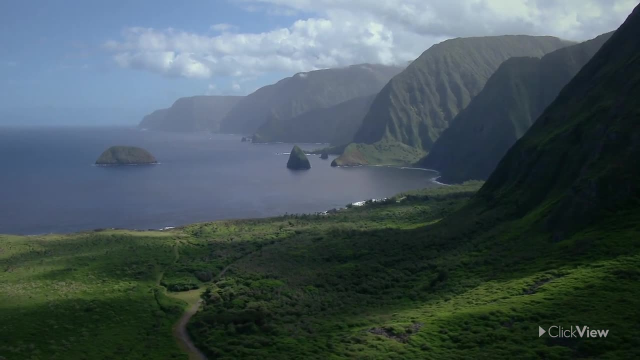 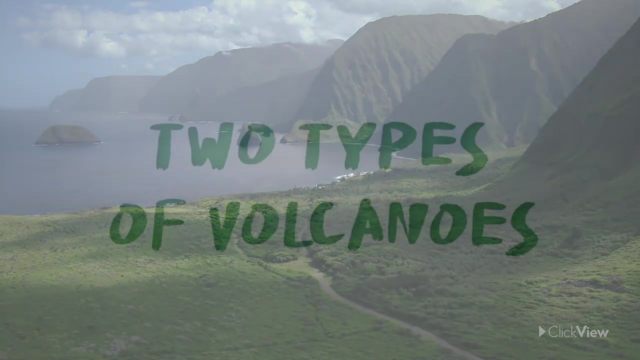 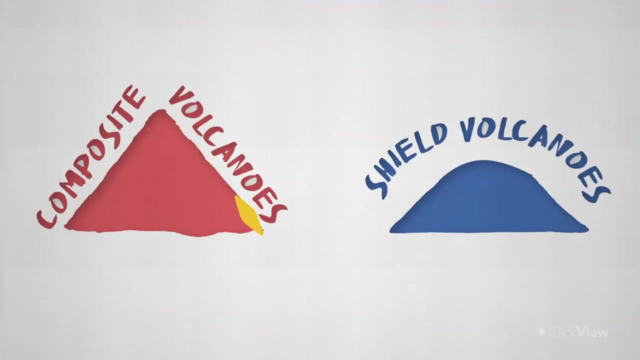 An example of this is the Hawaiian Islands, which are all made of a mixture of extinct and active volcanoes that have broken through the middle of the Pacific plate. Now that you know where volcanoes form, let's learn about their different types. There are two main types: composite volcanoes and shield volcanoes. 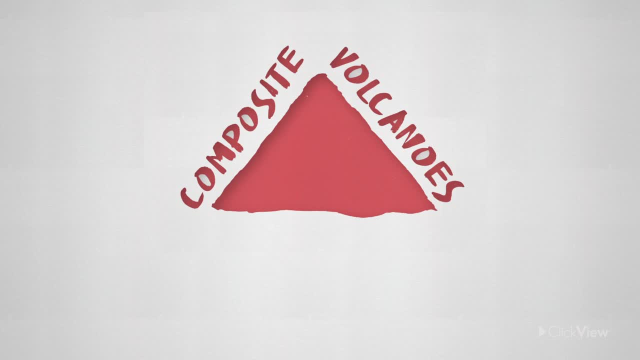 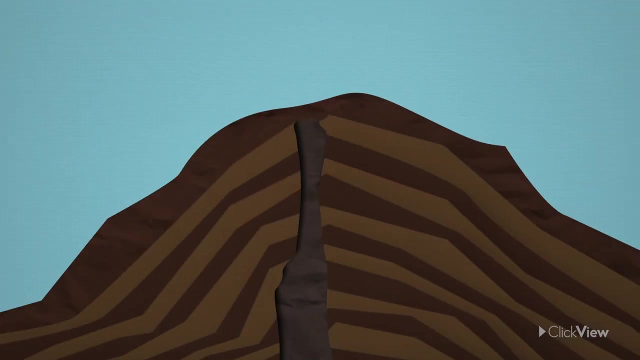 The majority of volcanoes are made up of a mixture of extinct and active volcanoes. Most of these volcanoes are composite volcanoes. These are commonly found on destructive plate margins and have a distinctive conical shape. Let's slice a composite volcano in half to learn more about it.